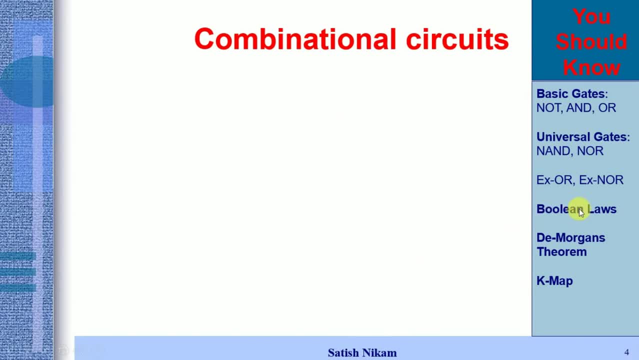 of all, the gate. you also must know about boolean laws, de morgan theorems and kmap. now we start the combinational circuit. if we observe this block diagram, combinational circuit is nothing but the connection between the logical gates to get some specified output without any storage means: the memory block. 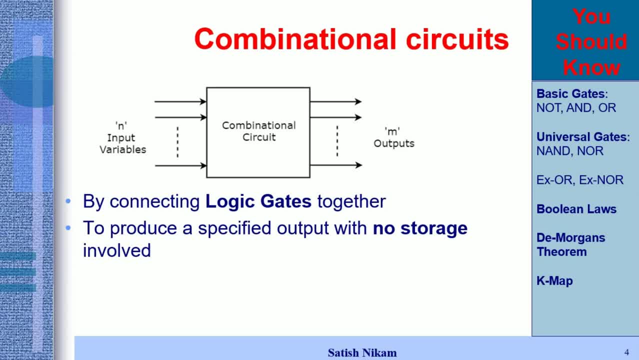 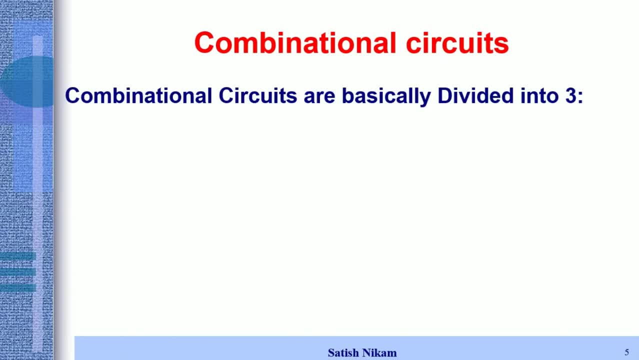 is not involved with the logic gates. so this type of circuit we call combinational circuit. basically, combinational circuits are divided into three parts: first one, that is, arithmetic and logic functional circuits. second one, code converters. and third one, data transmission. all these three types of circuits we are going to discuss in the 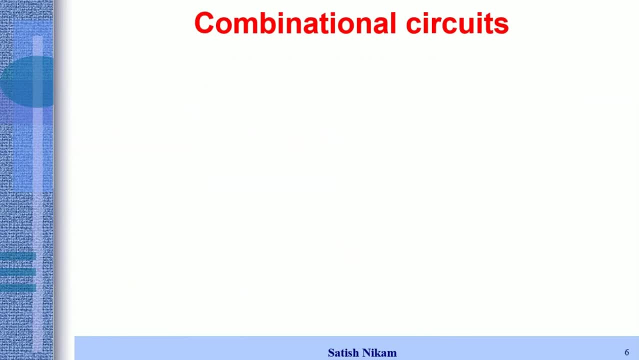 next part of this unit. now we have to design the combinational circuit. for the designing of combinational circuit we are having some steps. so design procedure of the combinational circuit is as given below. first one: we have to analyze the problem definition. then from that problem definition we have to find out the input variables and output variables. and 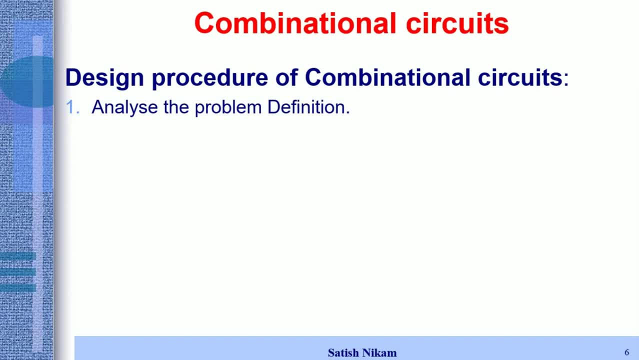 we have to assign the symbols for that: input variables and output variables. so we have to define the input variables and output variables. now, from this input variables and output variables, we have to formulate the truth table. to formulate the truth table is a very simple process. if n number of input variables are there, 2 raise to n number of possible maximum possible combinations. 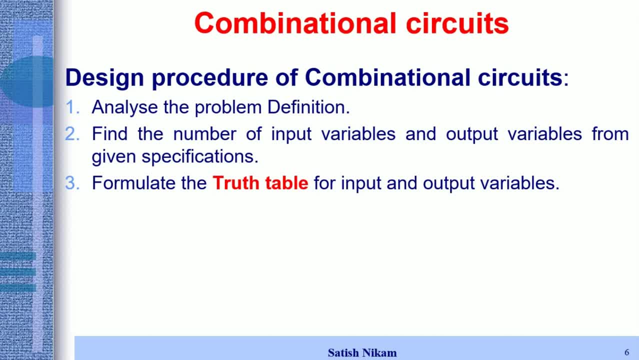 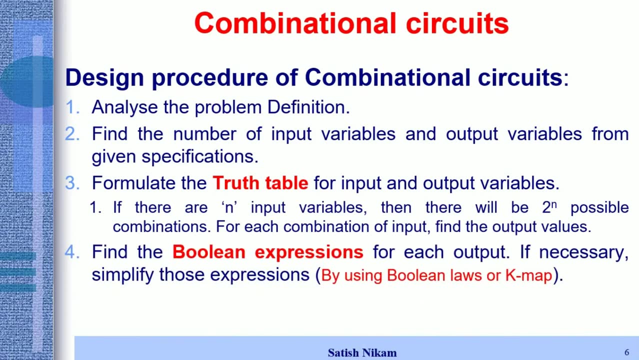 for the inputs are there and we are going to find out from the logic or from the problem statement what will be the output for that, every combination that we are going to write down. so that way we find the truth table And when we form the truth table, from the truth table we can write down the Boolean expressions. 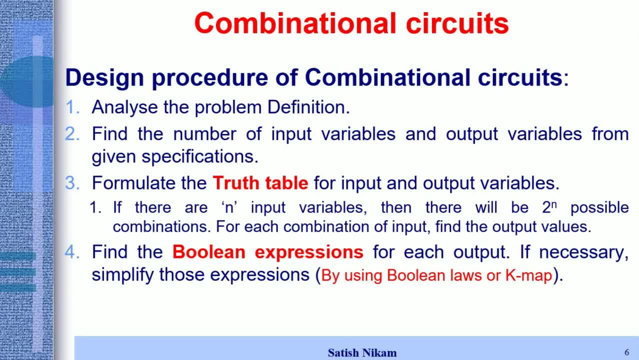 very easily for every input. for that purpose, we can use the Boolean laws or the K-Map technique, and when we got the Boolean expression by using the logic gates, we can draw or we can implement the Boolean expression for each output. so this is a simple design procedure. 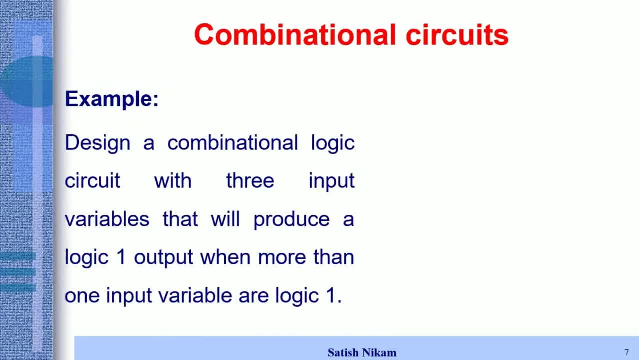 for the combinational circuits. We will take one example: Design a combinational logic circuit with a three input variables that will produce a logic one output when more than one input variable are logic one. so this is my problem statement. so from this problem statement we can write down the truth table. first step: 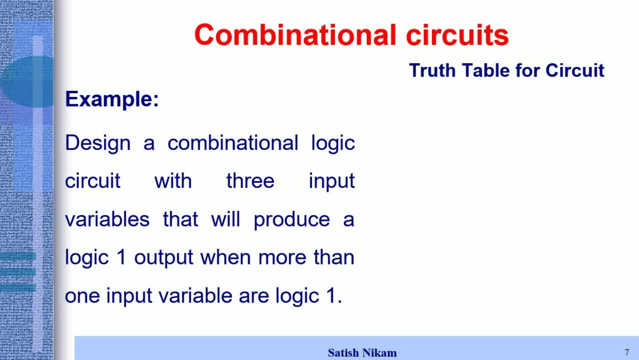 is we have to define the number of inputs and number of output. now from this problem statement we can say there are total three, number of inputs are there. we can say a, b and c And output is one, so that we can assign by y, so we can form here the truth table as three. 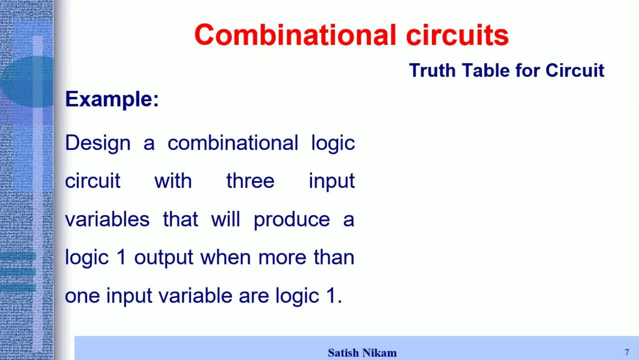 number of inputs are there. two raise to three. total eight possible combinations will be there in our truth table, so that combinations are: zero, zero, zero, zero, zero, one, zero, one, zero, zero, one, one, one, zero, zero, one, zero, one, one zero and one one one. these are the maximum. 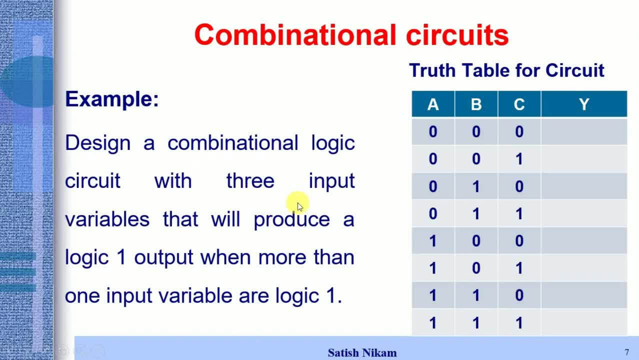 possible combinations for the three inputs. now from this problem statement we have to find out the output for every possible combination. in the problem statement it is simply given: when more than one input variables are high, output will be high. this is a problem statement and from that problem statement we can write down the outputs for every combination. now 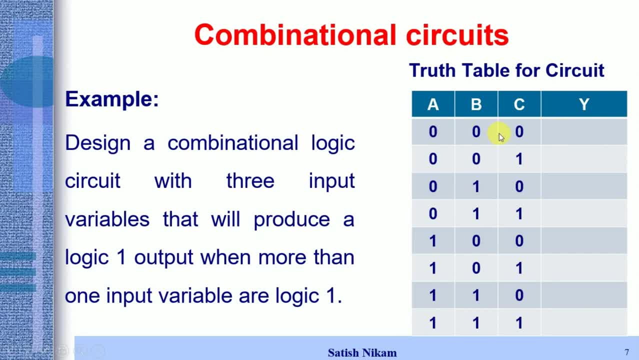 in the first combination we are not having any one input high, so definitely the output will be zero. Second, If one input is high, output is zero. only one input is high, output is zero. now in this case we are having two inputs high, so definitely we will get the output one here again only. 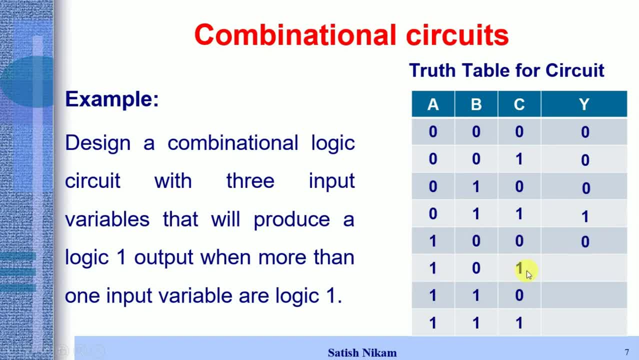 one input is high, we get zero. two inputs are high, so definitely we will get one here again in this. two inputs are high, output will be high and as more than two inputs are high, definitely we will get the output high. so we got here the truth table. now, from this truth table, 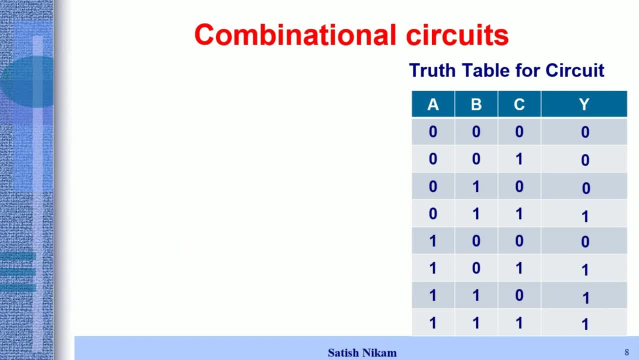 we have to find out the expression boolean expression. so for that purpose we are using here the k-map. as the number of outputs are only one, y is the output. so definitely we will have only one k-map. and as the number of inputs are three, two raise to three is. 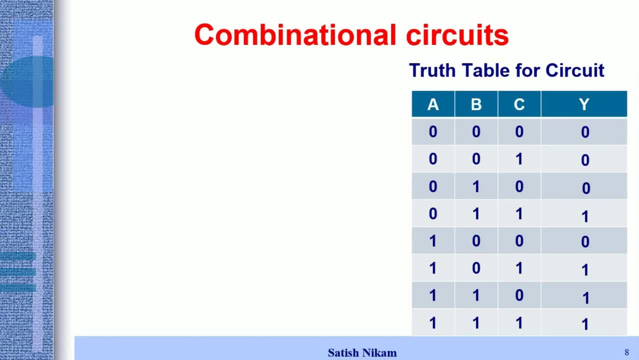 equal to eight. so eight number of cells should be there in your k-map. so we are going to draw the k-map From this truth table. so here for the y, we are having here the k-map, having eight cells, we write here: a, b, c a bar, a b bar, c bar, b bar, c, b, c, b c bar. now we are going to fill. 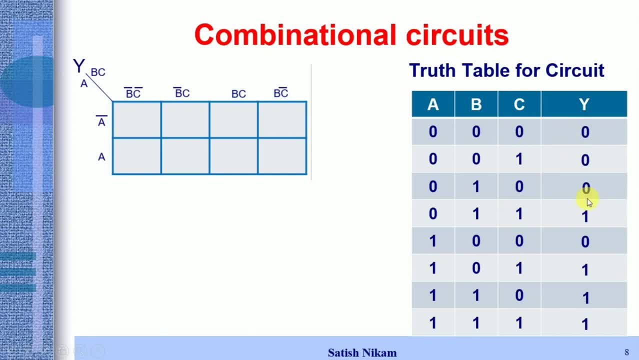 the k-map. a very simple technique is there? zero, zero, zero one. we write down here: zero, zero, zero one, and after that zero one, one one. we write zero, zero, one and after that zero one one. If you fill like this, we will get here the or we can fill here the k-map. so this is the. 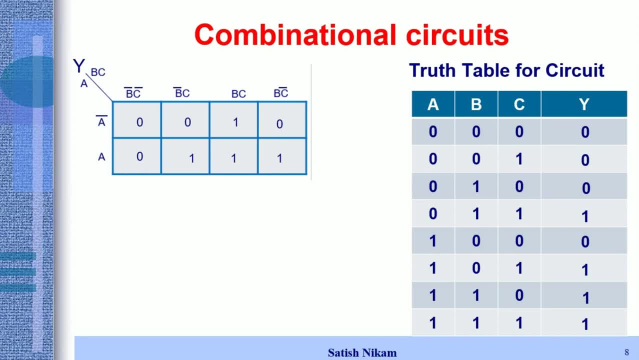 step which we have finished, to plot the k-map. now we have to form the groups, so we can form here the group of these two ones. next, we can form the group of these two ones and we can form the group of these two ones. this part we have already discussed at the time of solving. 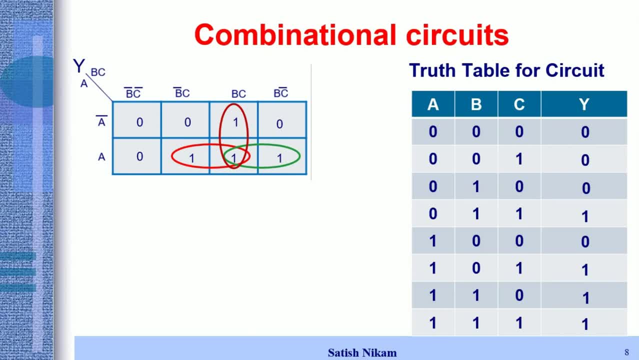 of a k-map. Now from this k-map, from this group, we can write down the expression. Now it is very simple technique to write down the expression from the groups, The terms which are constant, that we take and the terms which are. 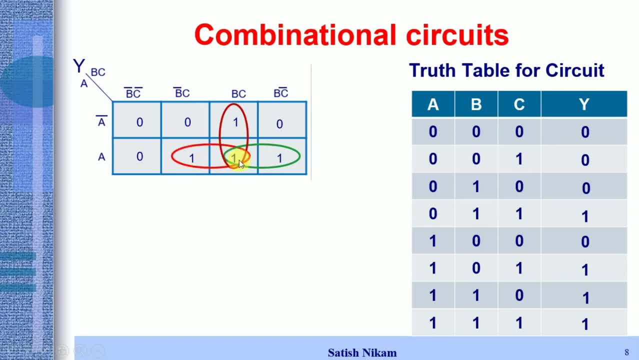 changing. that we neglect Now in the first group, if you observe very correctly, A is constant, C is constant but B is changing. So we are having expression here: AC for the first group. For the second group, A is constant, B is constant but C is changing. So we neglect C.